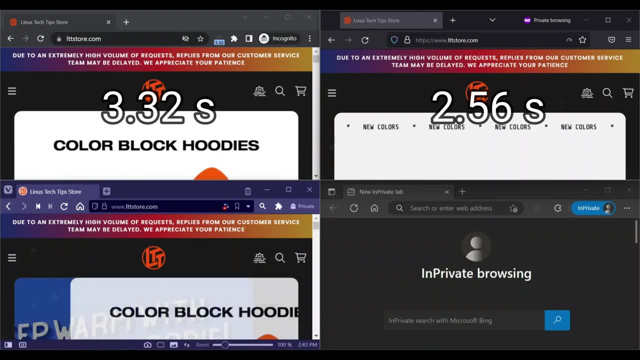 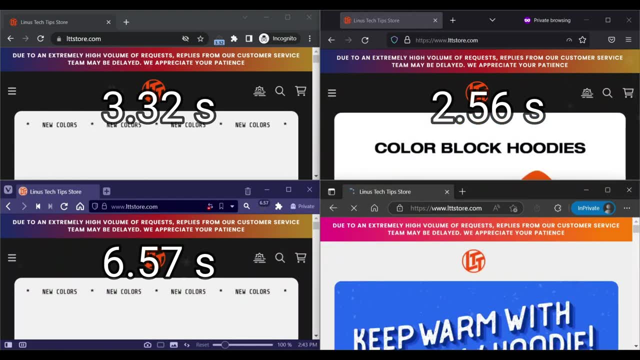 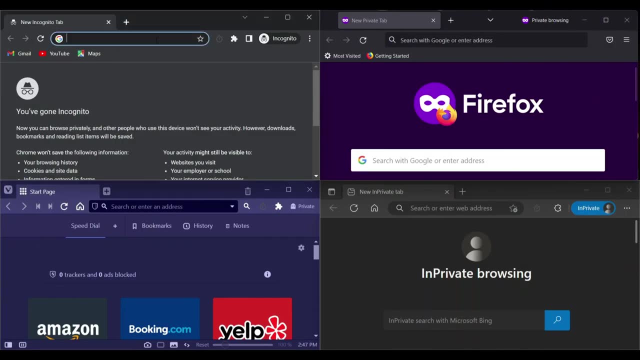 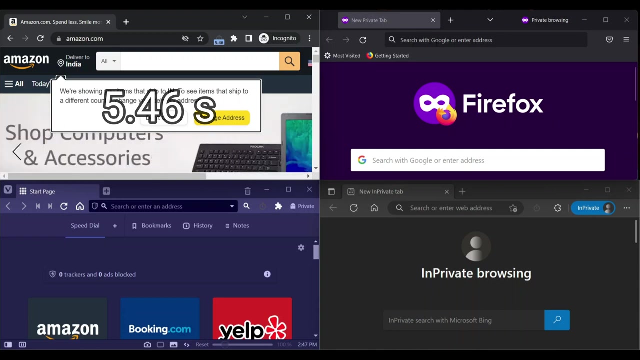 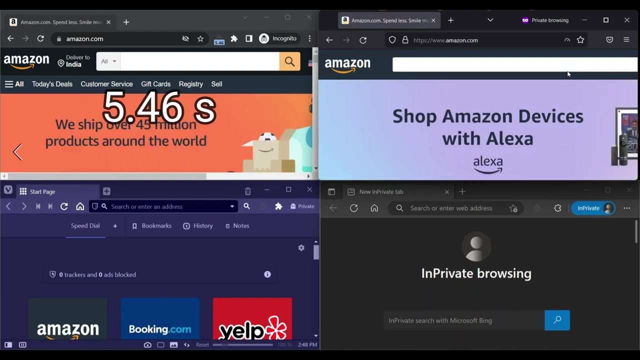 Vivaldi loads in 6.57 seconds. Edge loads in 5.11 seconds. Next website is Amazon. Chrome loads in 5.46 seconds. Vivaldi loads in 5.43 seconds. Firefox loads in 1.76 seconds. 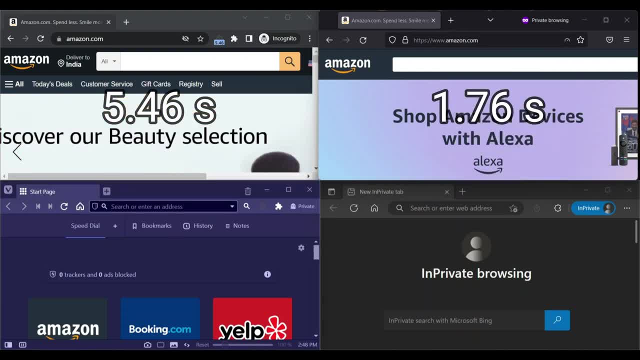 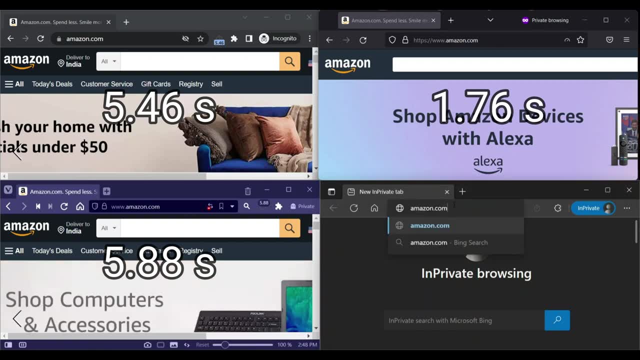 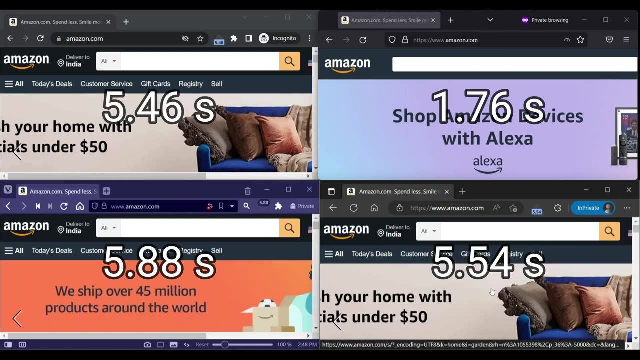 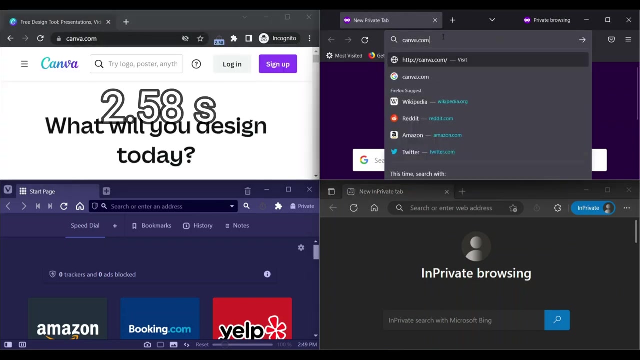 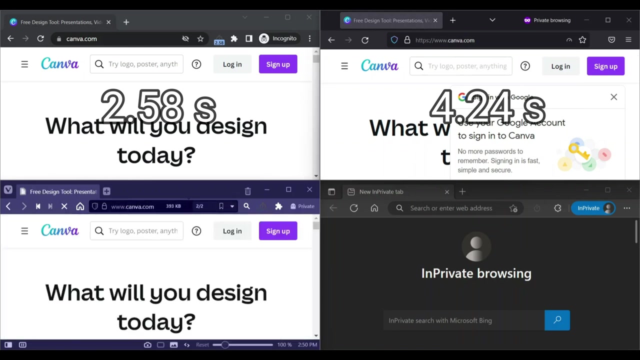 Firefox loads in 1.76 seconds. Vivaldi loads in 5.88 seconds. Edge loads in 5.54 seconds. Next website is Canva. Chrome loads in 2.58 seconds. Firefox loads in 4.24 seconds. 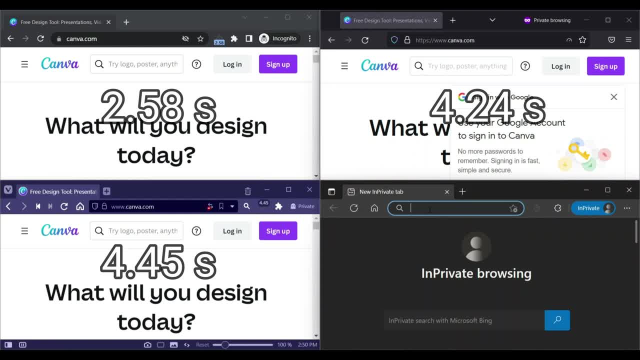 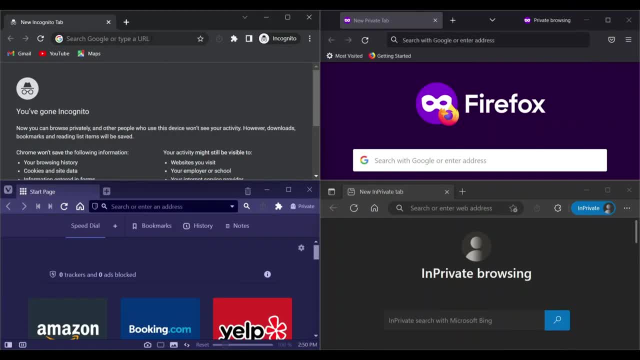 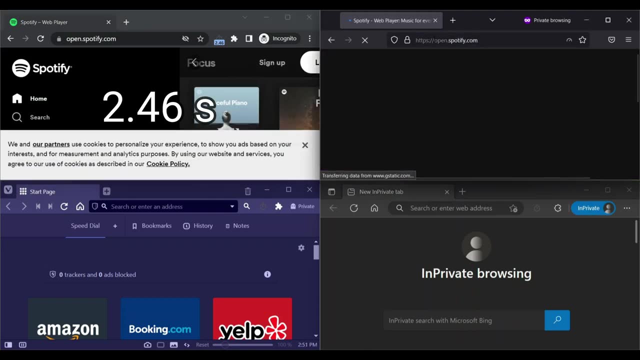 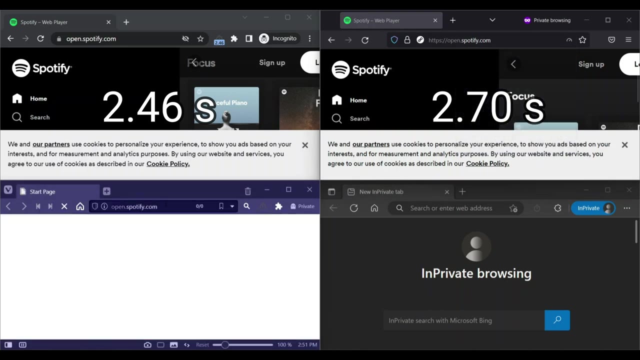 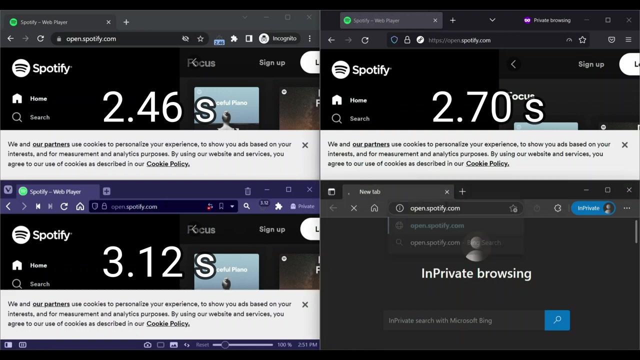 Vivaldi loads in 4.45 seconds. Edge loads in 4 seconds. Next website is Spotify. Chrome loads in 2.46 seconds. Firefox loads in 2.7 seconds. Vivaldi loads in 3.12 seconds. 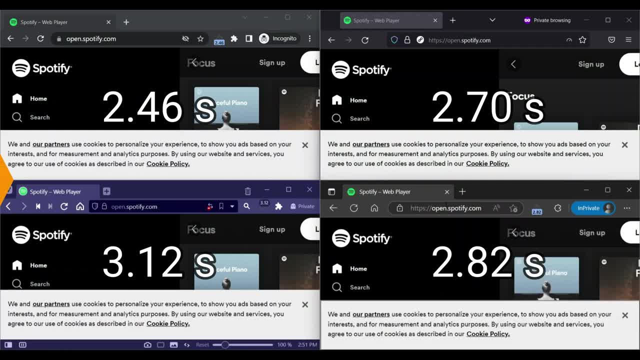 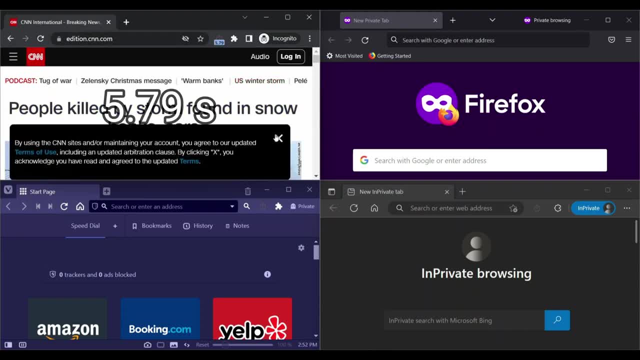 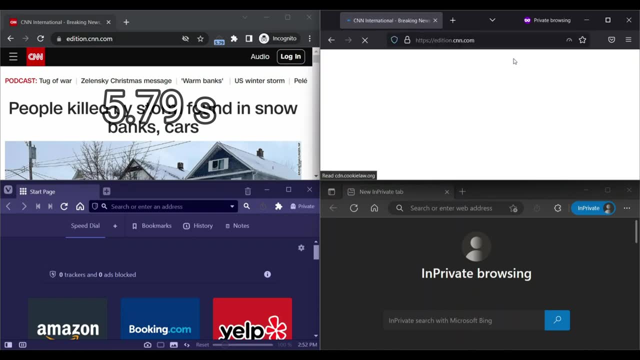 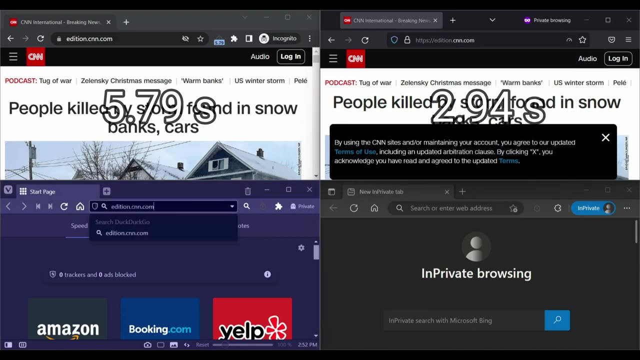 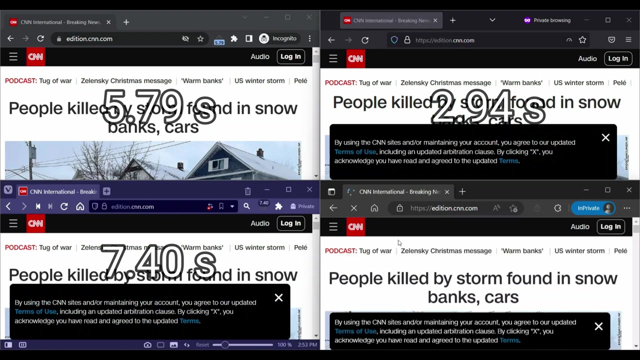 And Edge loads in 2.82 seconds. Next website is CNN. Chrome loads in 5.79 seconds. Firefox loads in 2.94 seconds. Vivaldi loads in 7.40 seconds. Edge loads in 7.45 seconds.